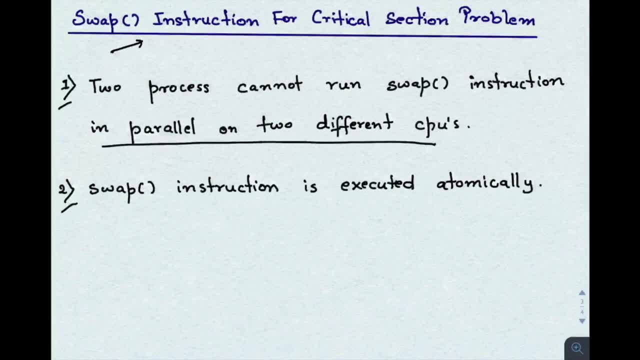 instruction in parallel on two different CPUs. So this is the first guarantee by the hardware. So this instruction can be run by only one process at a time, Only after that process I completed this instruction, then another process can run this, And also SWAP instruction is executed atomically. So that means once SWAP starts executing on the 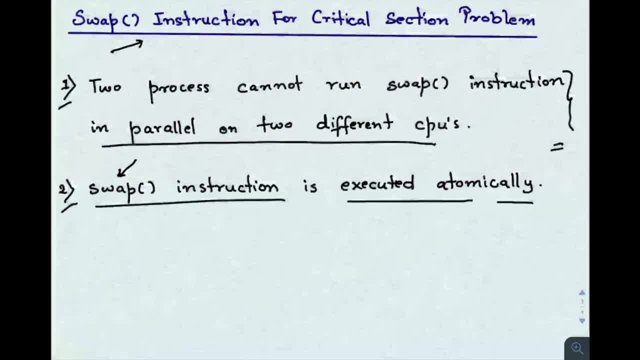 CPU, then it cannot be interrupted. So this SWAP instruction will have some lines of code right And in between. when the CPU is running these codes- line 1,, 2, 3,- it cannot be interrupted in any of these lines, Only after line 3 is completed. 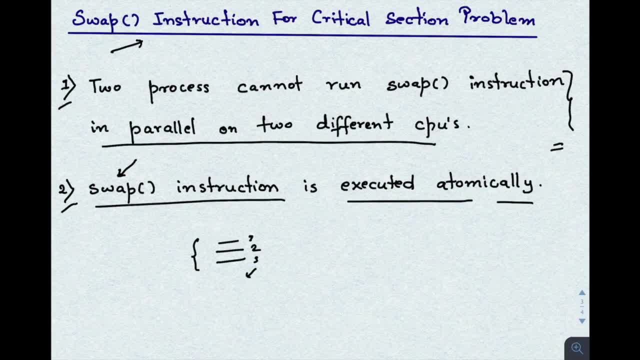 And after that, and this instruction completes finally, then only this can be interrupted, not before that. So we already know that two major reasons of the erase condition, if you remember. the first one is parallel execution. If you have parallel execution, 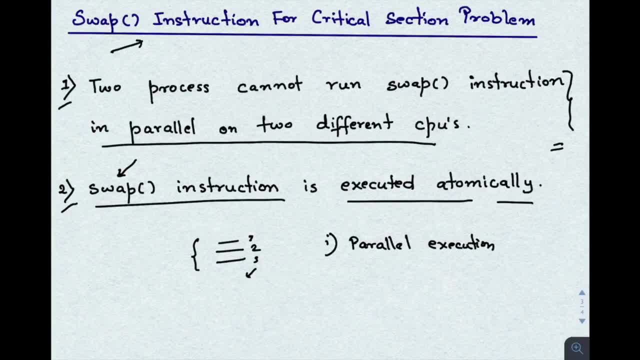 on different CPUs the same serial resource, using access on different CPUs at the same time. then erase condition can happen. And second is due to interrupts. These interrupts can be I mean hardware interrupts or interrupts by the scheduler itself, or it schedules some other process, And we have taken care of both these issues here. 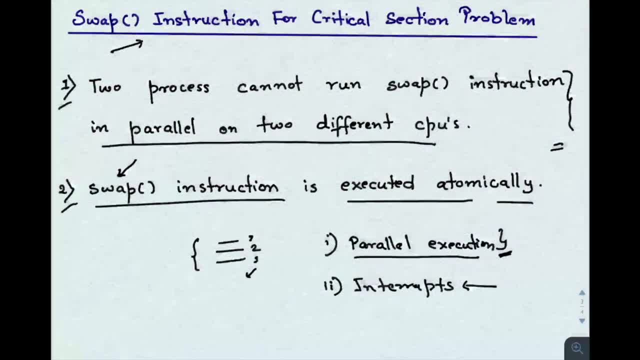 So parallel execution, I mean parallel execution, right? So hardware already guarantees that the SWAP instruction cannot be run parallelly on multiple CPUs. And also the second one, it is that instruction is executed atomically. That means that it cannot be interrupted by. 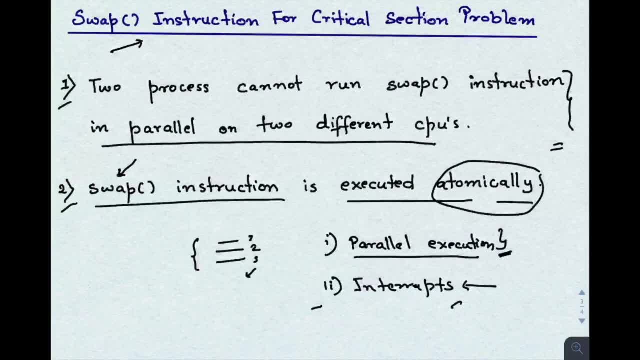 any other interrupts. So this is the first one, And the second one it is that instruction is executed automatically on multiple CPUs. so it's not an interrupts or any process. It cannot be interrupted. So we are avoiding both the reasons that lead us to the erase condition. 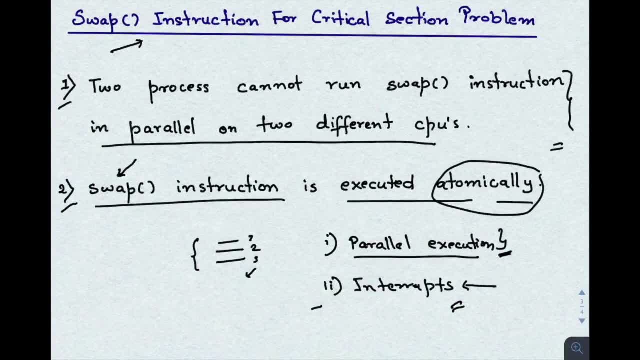 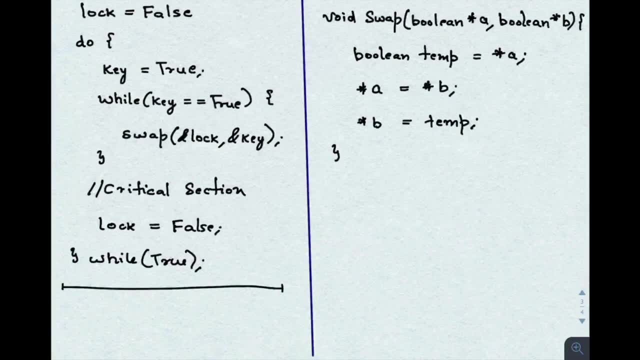 Now we will look into the critical restriction solution using SWAP. This is the solution- critical restriction solution using the SWAP instruction- and then I have defined the SWAP instruction separately. So what it does is it takes two Boolean variables. 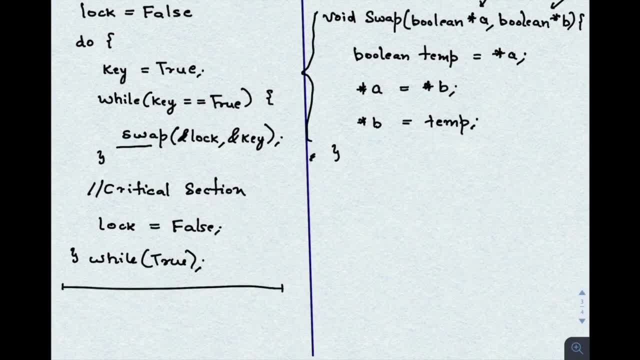 a and b and just swaps them them. so this function swap does nothing, it just swaps them. so another thing you should notice we have we are passing these variables a and b, boolean variable a and b by pointers. so this is. i mean, normally this is called by pass, by reference. if you see, here we have ampersand, here log ampersand. 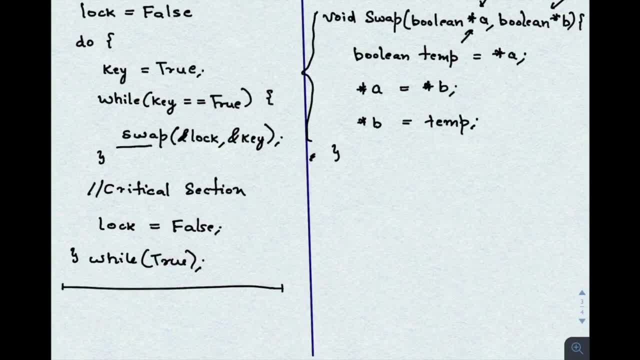 key and we have star a and star b. so this is called pass by reference. so in my pass by reference what happens? so if you change the value of a here and b here, that will reflect, i mean change of value of a will be reflected in the variable log here and the change of variable b will be reflected in the. 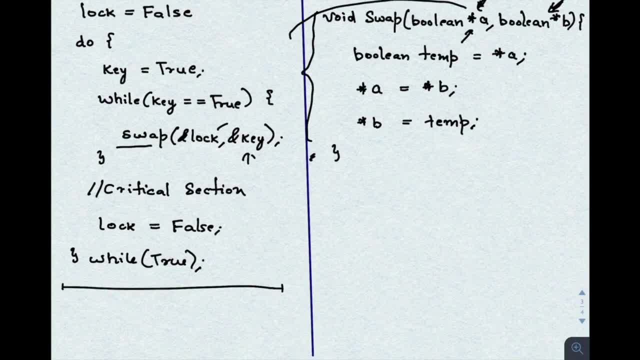 key here, and if you do not pass this by reference, if you pass it by value, you won't use ampersand and this pointer then i mean log and key. the changes that you make to a and b won't be reflected in log and key. so that's the reference and you can read more about. 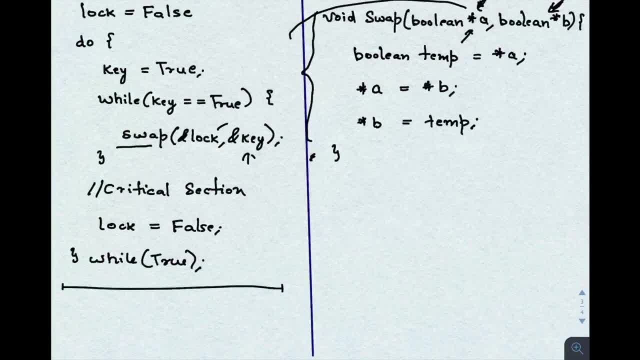 how to do this in the next video. pass by reference is done using pointers. you can. there are many links available online that can teach you about this, so i won't go in details of this. you just you should just remember that any change you that you make to a will be reflected in the log. any change you make to b will be. 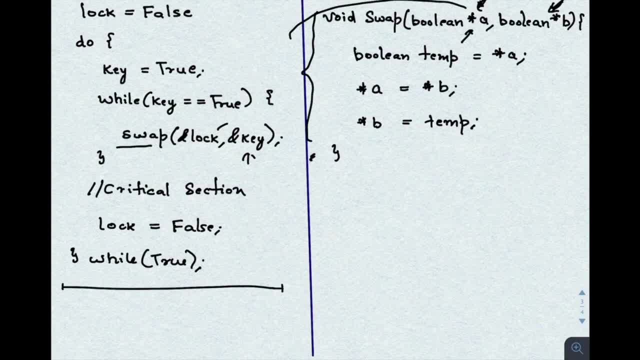 reflected in key. so what you are doing is you are interchanging the values of a or a and b, so that means you are interchanging the value of log and key. you are just swapping log and key. that means, if let's say initially, log is- equal to true. 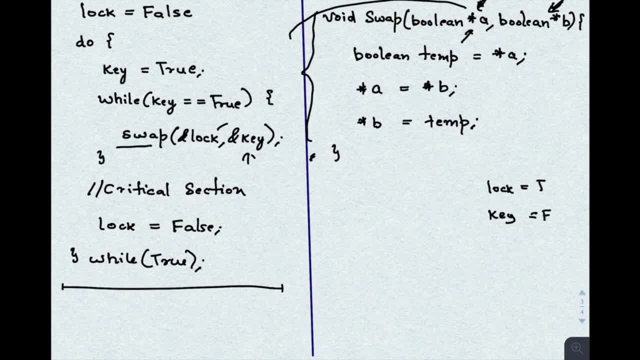 and key is false. right, this is the case initially. so initially, log is false, let's say, and key is true. let's say: and if you pass this, use the swap, then pass this log variable false, then give the swap function. so after swap executes, the output will be- i mean not the output- the value of 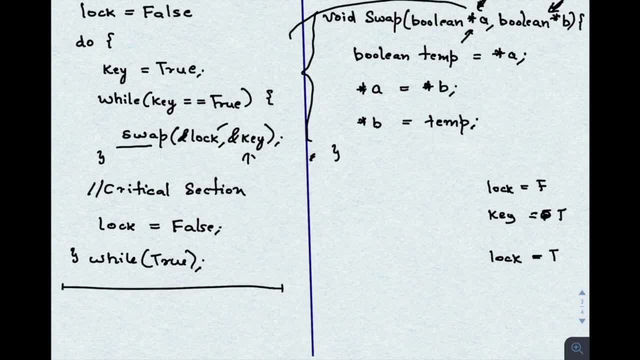 log will become true and key will become false. so that's this, when here and just swap both of this, that's what happened. so this is the and this is a simple thing that swap does and, as as i have already told, this swap this whole lines of code, three lines of code is. 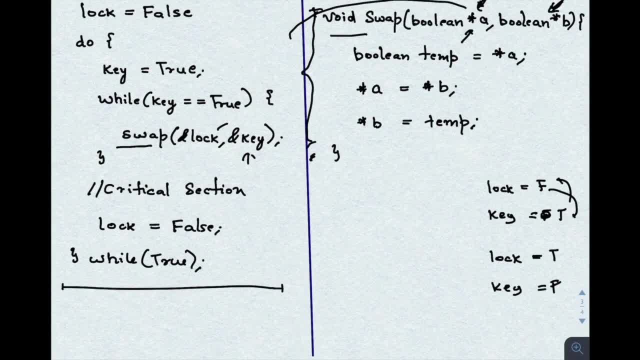 guaranteed to run atomically. that means it cannot be interrupted between i mean here or here. so only after this third line completes and this instruction completes completely, then only this can be interrupted, not before that. and another guarantee was that, uh, yeah, so another guarantee was that, okay, we will talk about mutual exclusive, then we will talk. another guarantee by the hardware. 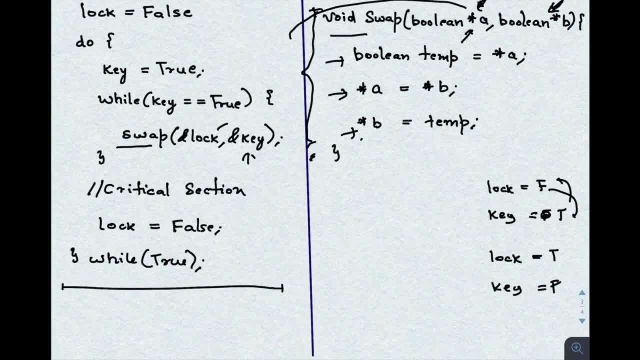 now let's look into this code. so initially, okay, now you've got this. okay, first understand this. wild cases: true, right. so if any process has to enter this critical section, it has to make this. while i mean false, right, while false, then only this can the while loop will be broken, and then 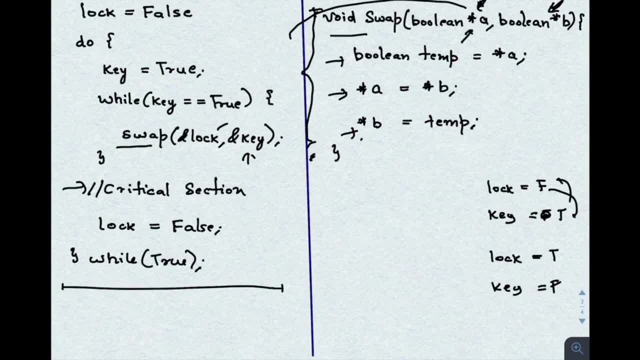 the process can enter critical section. so your aim should be so. any process will try to make key equal to false, right, then only it can enter the critical section. this is the aim of process: to enter the critical section now. now remember one thing: whenever a process enters this, it will set. 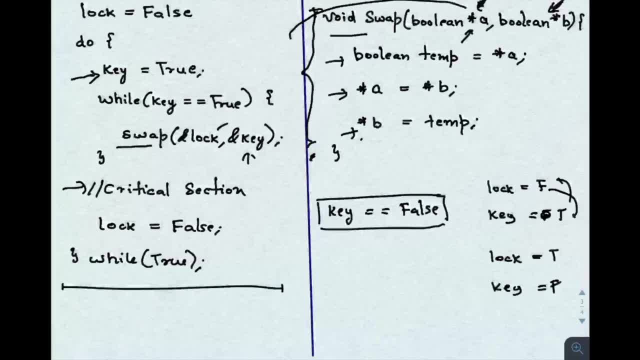 the key equal to true right, and the only way of making key as false is when. so when you go into this, while you are swapping this right lock and the key- but you already know that with i mean when a process enters this- the key is true right. so the only way of making key as false is when lock is. 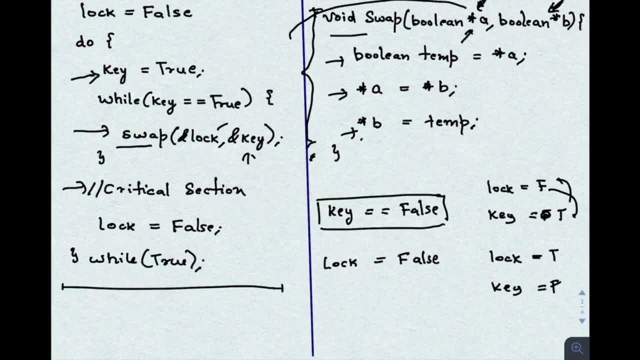 false right. so when lock is false right and and you do the swap this thing right, swap key is true and lock is false, then only lock will become true and key will become false. and once lock is true, admins. uh, so this has acquired the lock and now, since lock is true, admin, it can enter the critical. 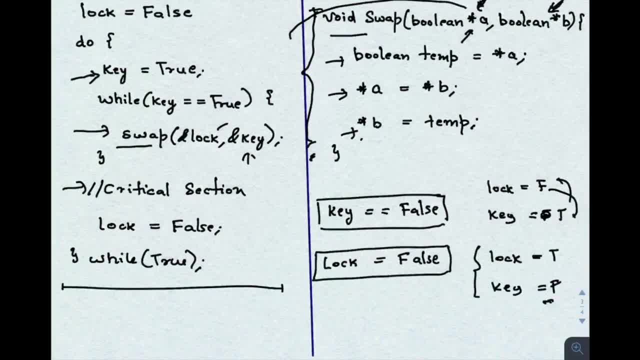 section. so that's what you should understand about this. so it's very easy to understand. you can uh, take any uh p1 and p2, and you can, i mean, try running this code. the only laws you should remember is that this uh. okay, now let's go into the mutual exclusion thing. uh, mutual exclusion. 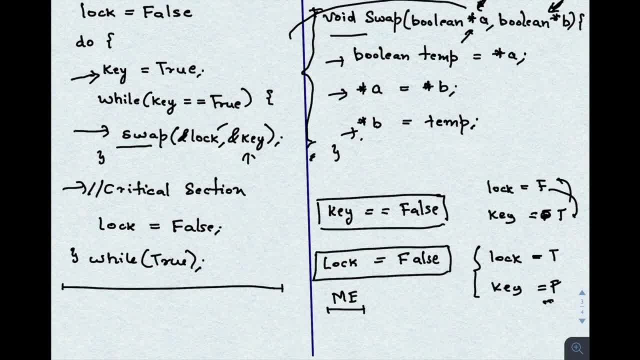 right. so, as i have already told, told, let's say, even if you have processed p1 and p2, both, uh, make the key as true. let's say, now both try to enter this while loop. now both will see key as true, both will enter here in this swap instruction. but you know that swap instruction. 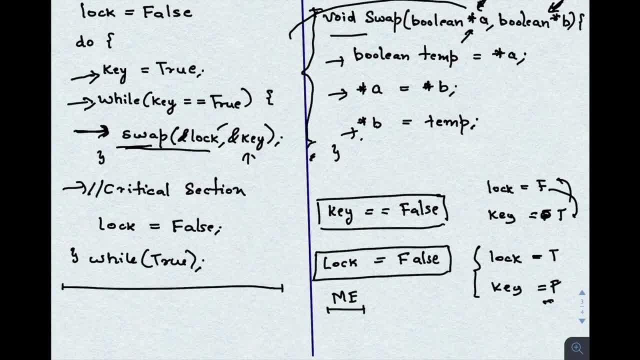 can be run. it cannot be run parallelly, so only one of this p1 or p2 will be able to run this first. so that is so. we do not know which one p1p that is now we're taking care of by the hardware. you can run this first. so that is so. we do not know which one p1p that is now we're taking care. 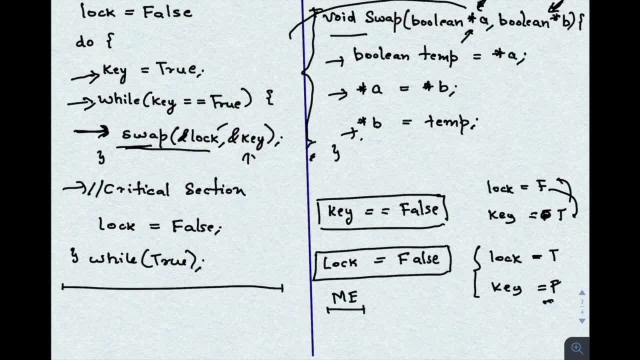 any order can be: either p2 can run this first or p1, but they cannot run it parallelly. so i mean any one of them will be able to set the, i mean swap this, and make the value of key as false, and then it will even able to enter the critical section. so you are. so this solution satisfies. 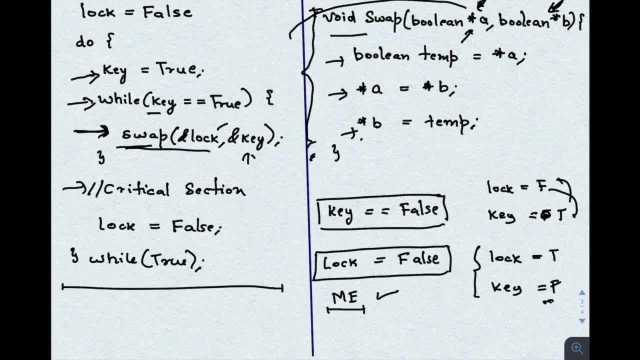 the mutual exclusion and also deadlock cannot be here. so, as i, as i already told, even if both of them enters here- and we already know that i mean lock can be either true or false right. so i mean, when it is true, that means one process is already in the in the critical section, and when 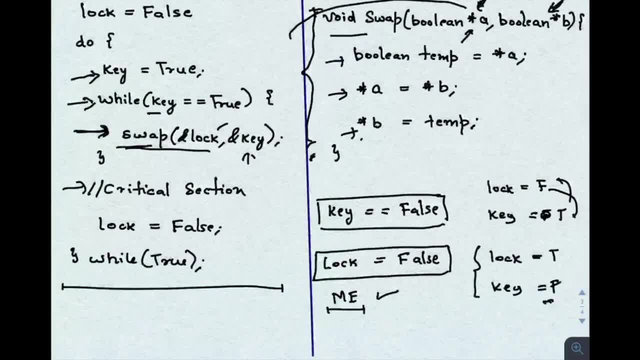 it is false. that means that one process will be able to enter it. so that is deadlock. cannot happen here. and let's look into the progress requirement. so progress you can easily check is first allow let's say p1 to enter this critical section right and let it exit here. i mean exit, it exits here. 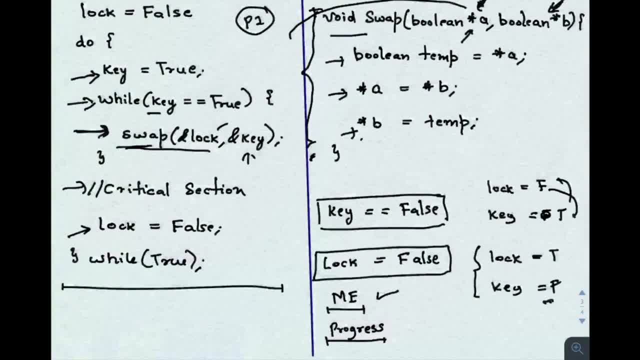 after this log statement. and then it wants to: let's say: you have reminder also right, let's. let's say it wants to sleep in this. a, probably, that is process p1. now let's take the case of p2. now p2 wants to enter this right. 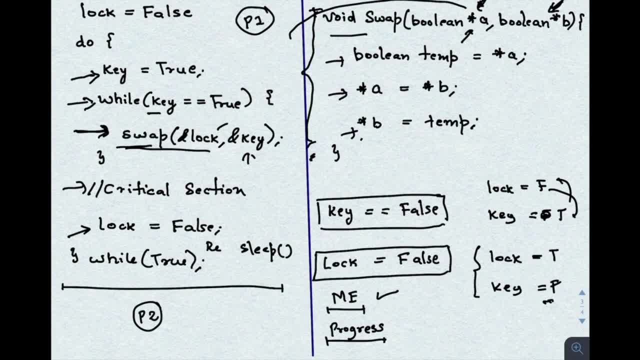 since when p1 exits this, it will make the lock as false right. so so when p2 tries to again- i mean access the critical section, then key will become false and it can access right and let's say again: so, p, so p2 has accessed this critical section first time. 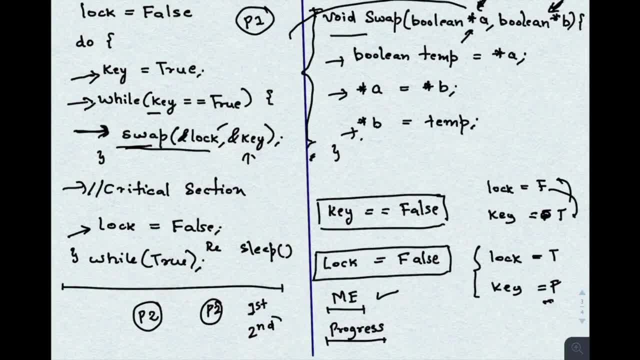 now let's say it again wants to access this second time, then also it can access, because p2 will make again- i mean, while it is exiting this it will make block as false. then again it can enter. so it's not happening that p1 is blocking p2 from entering again and again. right, so progress is satisfied. 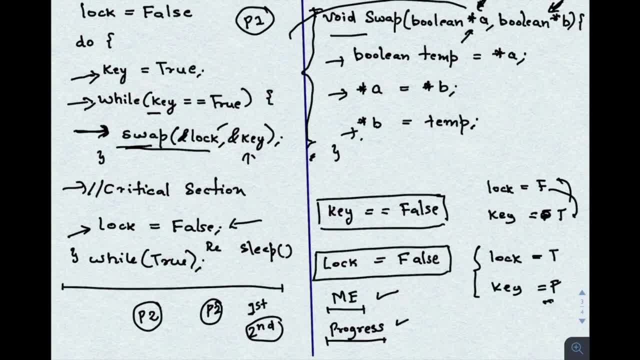 here, so progress will always be made. and another was a bounded weight, so bounded weight will not matter, so i ignored this restriction. so i will tell you once again the way you can, How you can enter this rest of this right form. So let us say so. if you see, let's check feeding out p1, so p1. 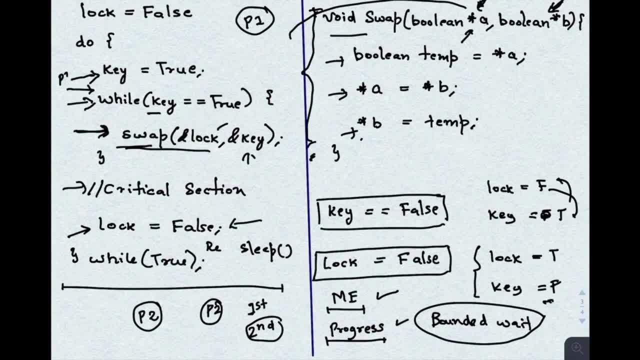 has, I mean, already gone through the Korea section and it again wants to enter this critical section and it is at the this while loop event and p2 less C is also waiting in this while. look, right now, is there any way that i mean there is no blocking off, like p1, like right even again can enter? right, there is. 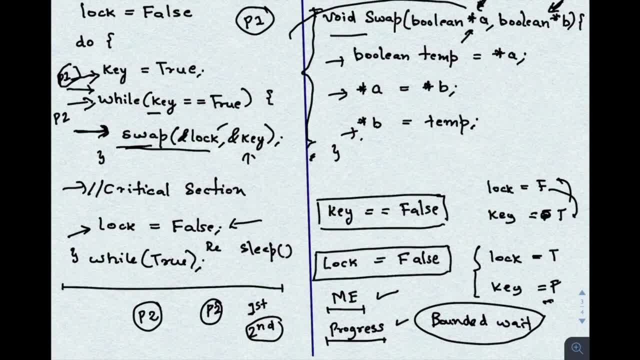 happen is p1 and p2 both try again to this swap instruction, right, and the hardware can pick up p1 again. so it's not guaranteed any order right that p2 will. since p2 was waiting first, it should get the. i mean it should run the swap instruction. so there is nothing like that. i mean hardware can. 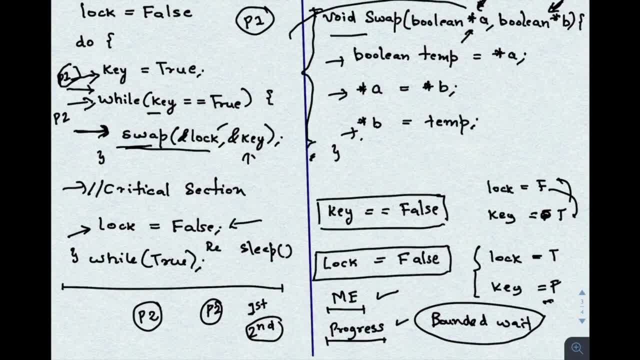 pick any any one of them- p1 and p2- and run it again. so there is no condition blocking p1 from running this swap again and again. so what can happen? p1 will keep on running this swap and entering the critical section and p2 will. i mean it can, it can happen, it it. it will be waiting in. 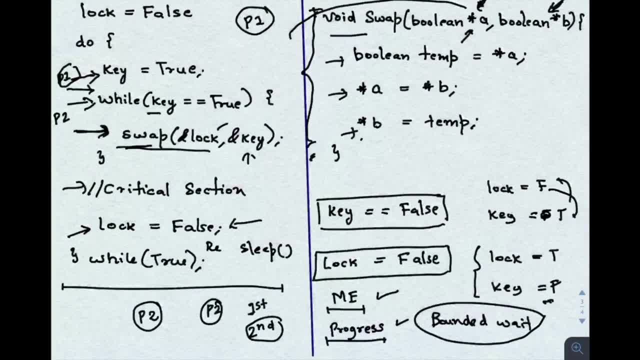 this while infinitely and it will stop. so it will not be able to enter the critical section forever. so that can happen here. so this does not satisfy the bounded weight, but this satisfies the two important requirements of the critical section problem, that is, mutual exclusion and the progress. 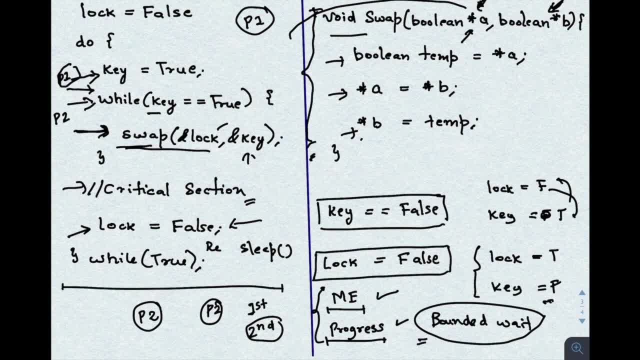 and the only issue is that this solution is not fair in the sense that i mean it does not guarantee the bounded weight. so one process can start, or multiple process can start there due to one of the process. so these are the two hardware instructions. so one is the test and set and another is the swap. so you can. 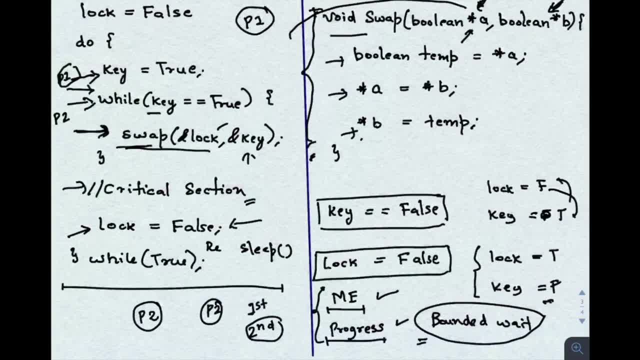 see that these two will be able to solve our critical section problem. and swap also has same issues as the test and set. one is the bounded weight, another is that this while loop right, so this is called, like you can, spin log. i mean in the sense that this while loop just wastage the.